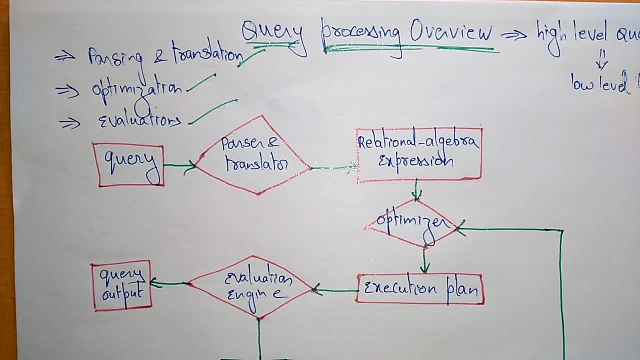 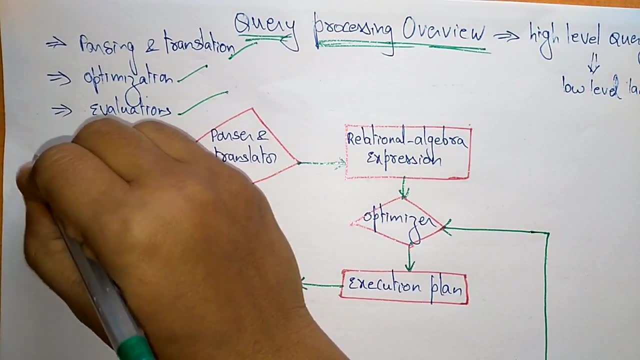 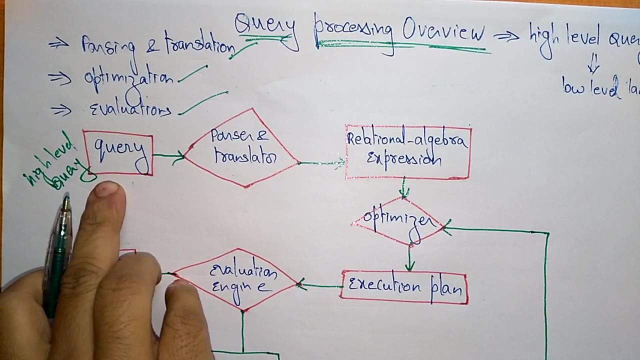 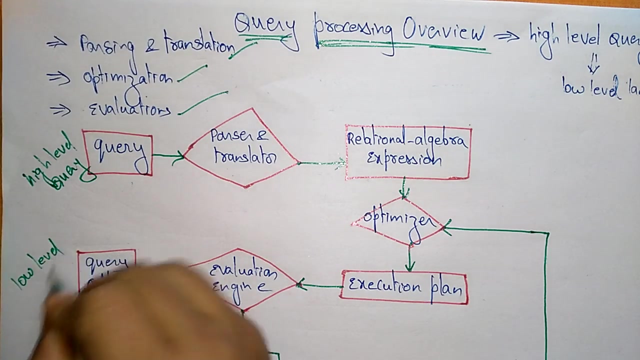 Okay, so these are the steps in query processing overview. So let us see in this diagram: The first is a query So which is in high level language. Hi, this is a high level. This is a high level query, So this high level query will be translated into low level language at last. So here you will get the low level language query. Okay, so here the high level query. first it. is the tax and then it is going to have an. Interestingly, this is a high level query. How to explain what a high level query? Well, it is going to be compared to the query we have just heard of the Torah in Yav erro. it. toutes the questions as A. Why did we do different types of curves? only so because we are using a three into four type, algebra Foresis. Next thing, we are referring to three Synonyms which can say: assets are quantity of property of a material in the form f. 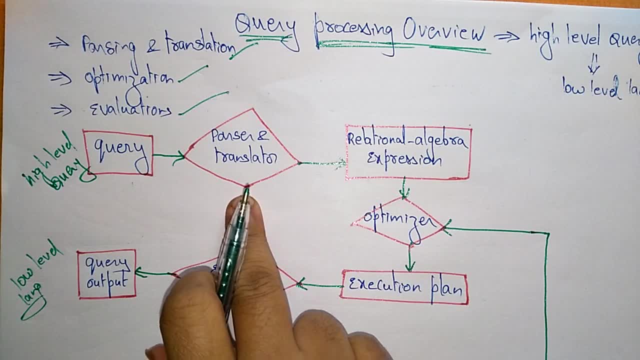 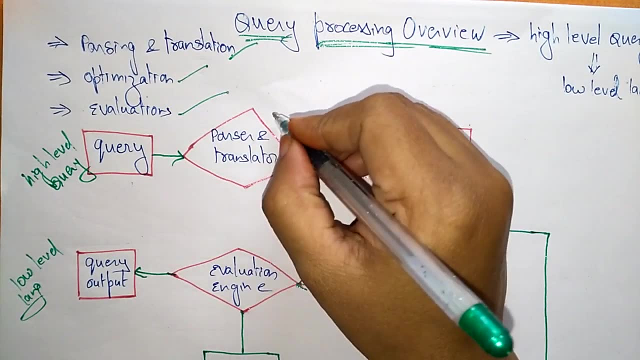 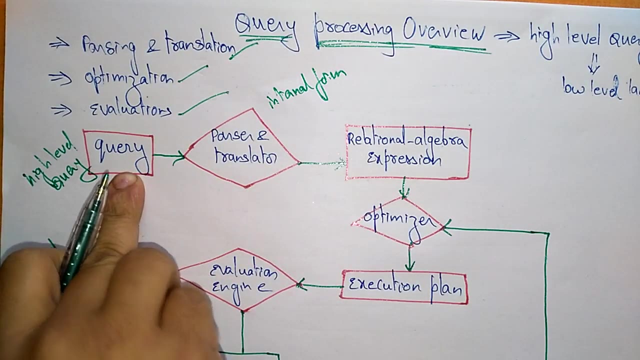 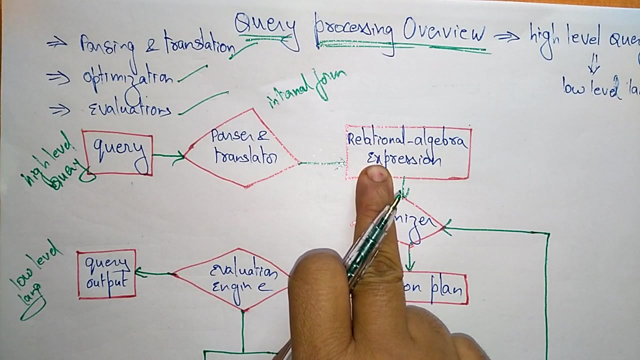 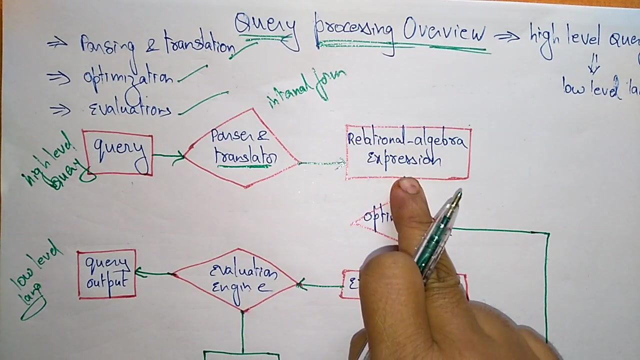 Then, excuse, Theicamente is case data is able to say that there is a called комна' aten and then translates into relational algebraic expression. okay, so the translator first converts the query into internal from and it translates to that relational algebraic expression whereas parser is. checks the. 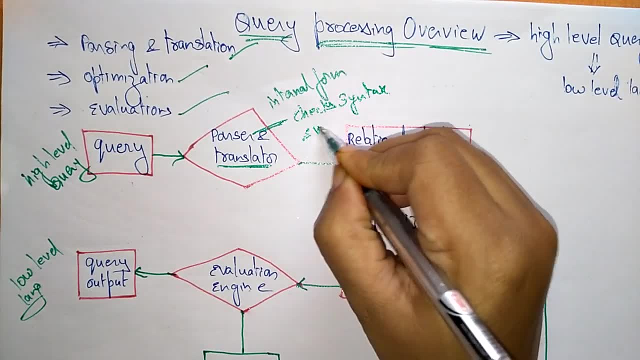 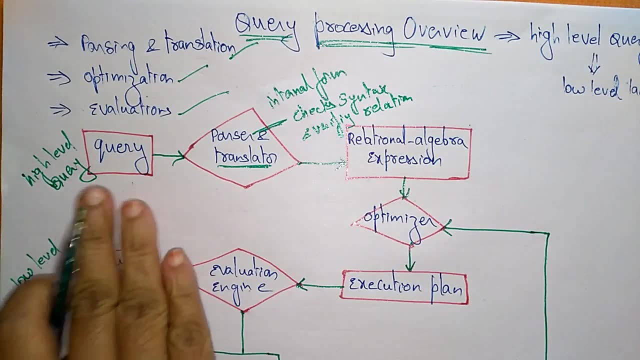 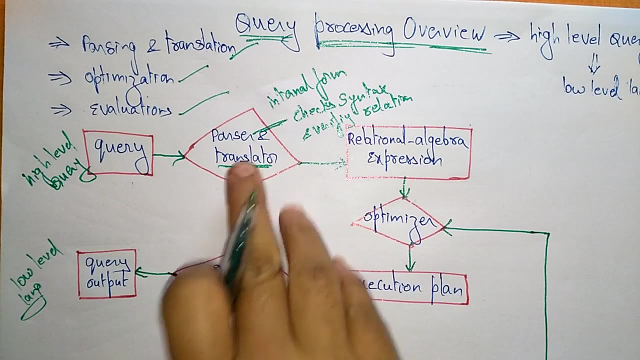 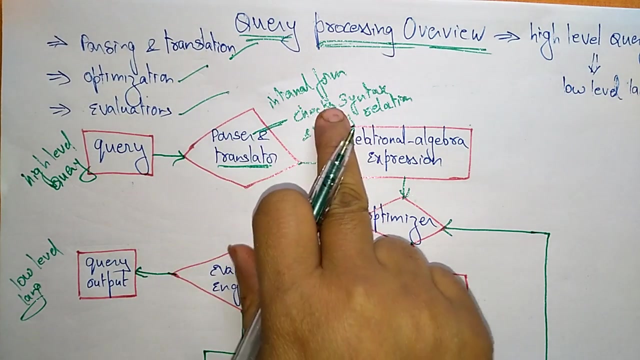 syntax and verify the relation. so that is a work of the parser. so first we are taken the query from the user and that query will be placed on the parser and translator. here the translator will convert the query into internal form, whereas the parser is used to check the syntax and verify the relation. so after that, 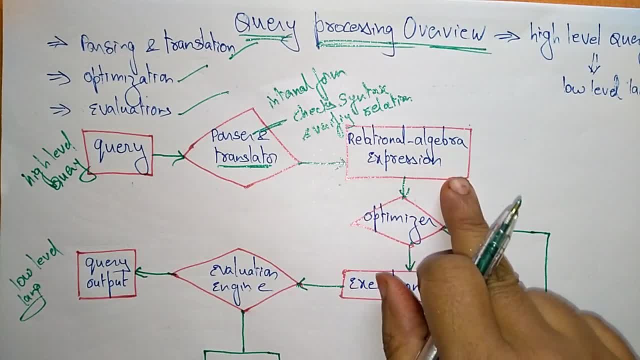 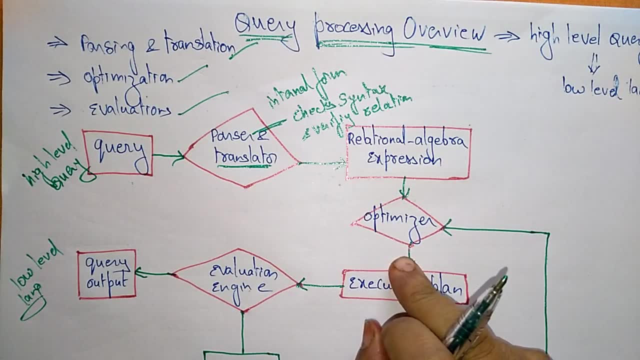 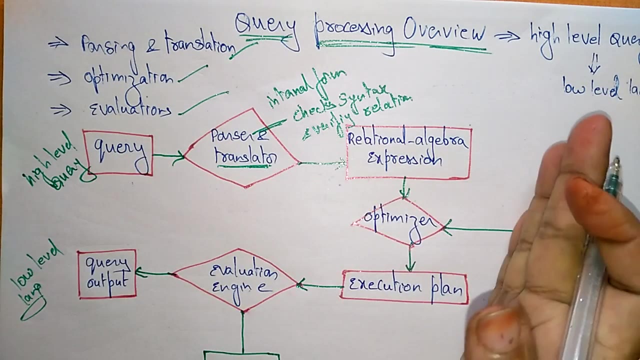 the expression enter into relational algebraic expression, so that relational algebraic expression- グ t licenss going into relational algebraic expression, の 결算力- will be sent into optimizer. so here what this optimizer will do. so, whatever the sql query we are given that now converted into relational algebra expression. okay, after that that relational 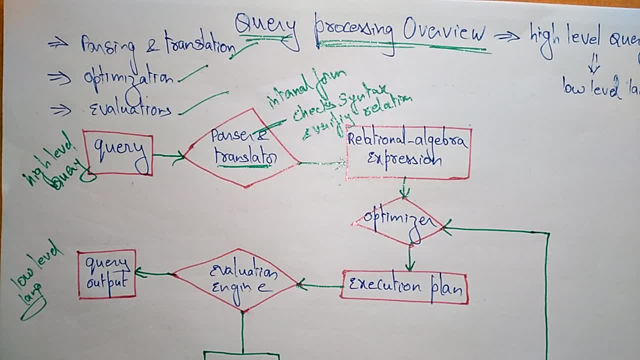 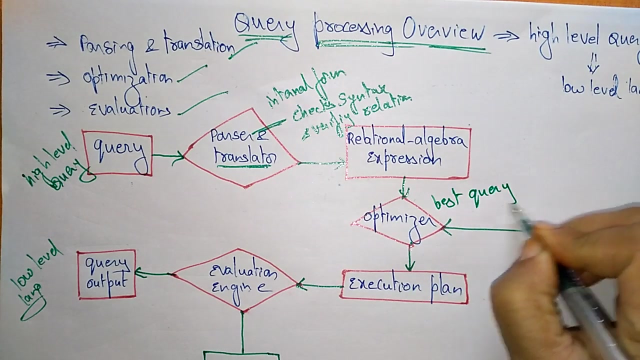 algebra expression will be optimized. optimization means it increase the performance of query by selecting the best query. okay, relational algebra will give two or more queries. okay. one, two or three more queries with the same equation: relation: okay. so in that this optimizer will select the best query. optimizer: select the best query, support a and b or two queries- okay. 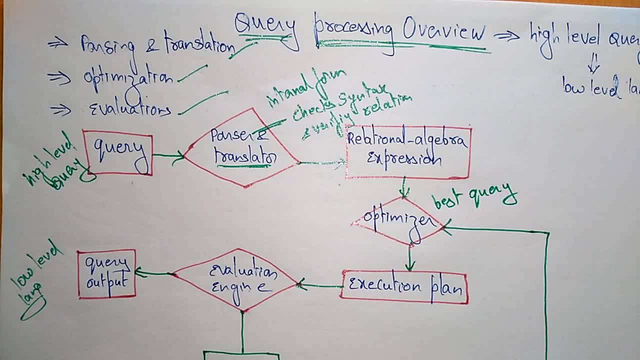 these two queries. here the optimizer will select the best in a and b. so then you can say a is optimized than b means. a is the best query when compared to b. so a is the best query when compared to b. so a is the best query when compared. 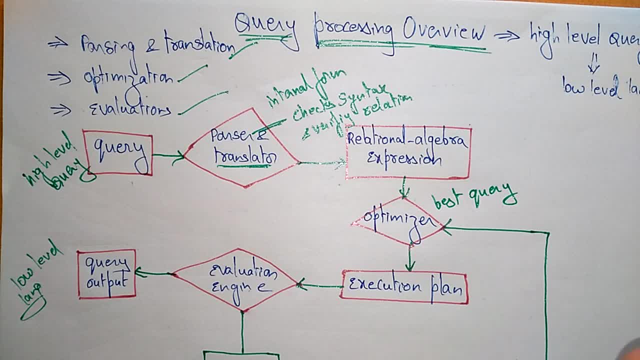 to be here. we are just comparing only these two. okay, we are not comparing entire database, only the relation between the, whatever the queries we are taken. okay, so that is related to relational algebraic expression. so the relational algebraic expression can be expressed in different ways? okay, in the different ways, different queries. this optimizer will select the best query. 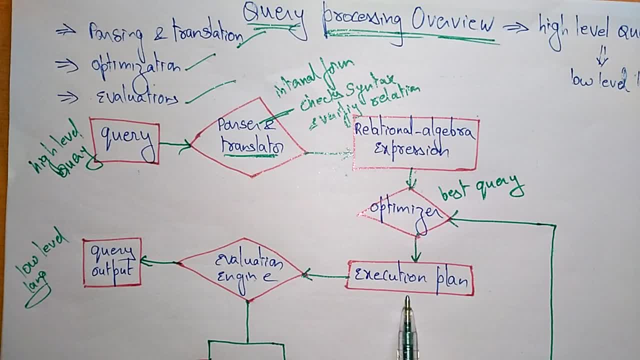 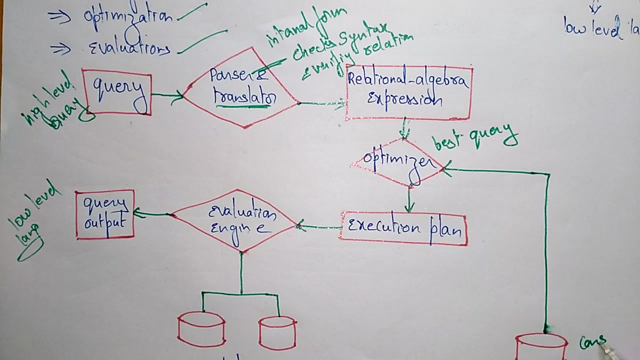 okay, and that will be placed on the execution plan. now the execution plan will execute. the engine takes the execution query execution evaluation plan and place it in on the evaluation engine. okay, so here the statistics and about the data this helps the it consists of. it consists of dbms catalog. 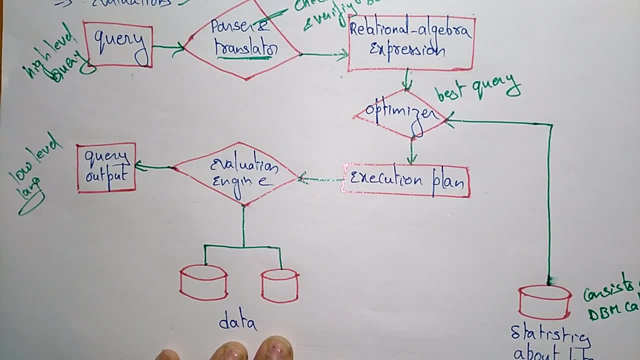 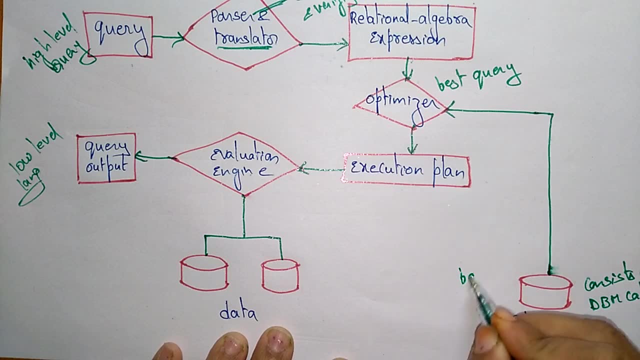 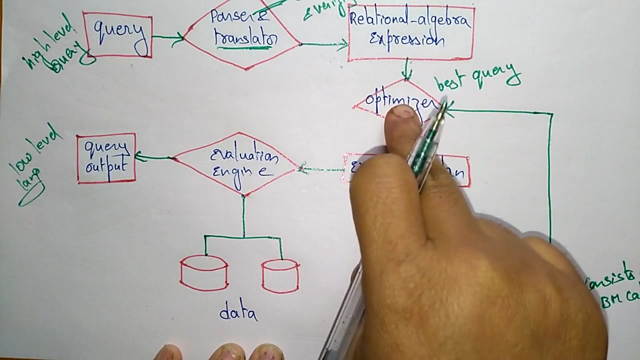 okay, so what the statistics about data will do? it is a metadata data about data. it is used for the best evaluation of query, best evaluation of query. so it helps the optimizer for best evaluation of the query. so, after evaluating the best query, that will be placed on the execution plan. now that execution plan. 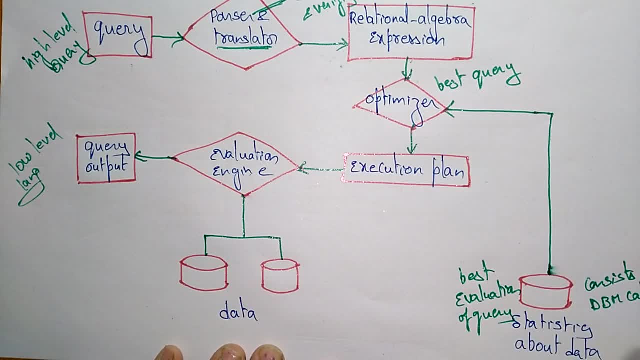 will send that plan in the form of it is in the form of a tree. okay, so query tree execution plan. always, the plan will be represented like it is in the form of trees, then only it will be understand. okay, so that execution plan will send it in the form of query tree. 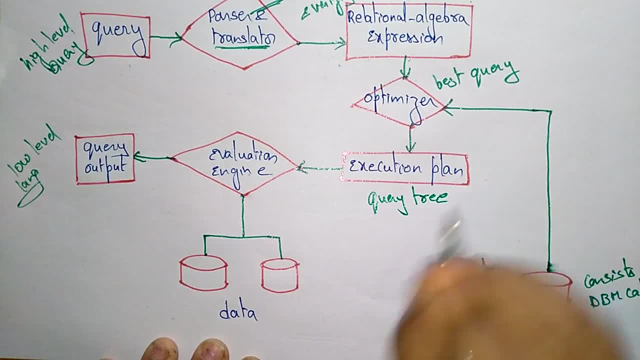 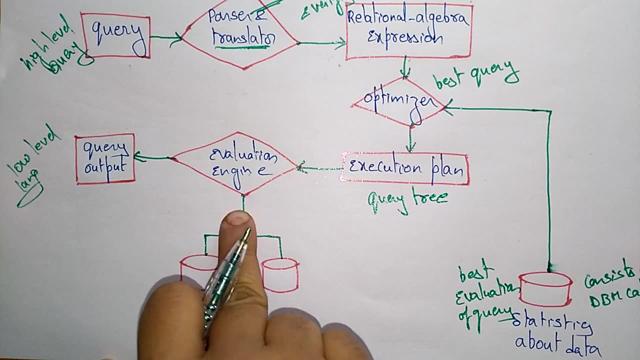 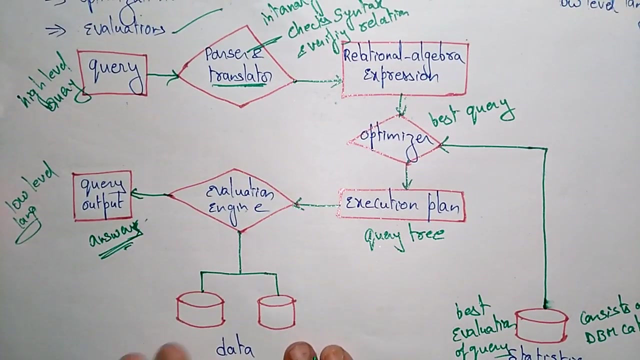 query tree and place that best query tree in the evaluation engine. Now the evaluation engine takes the best plan and returns the answer to the query output. Now you will get the best answer. okay, so this evaluation is engine is having the buffers like some data. extra data will be present. 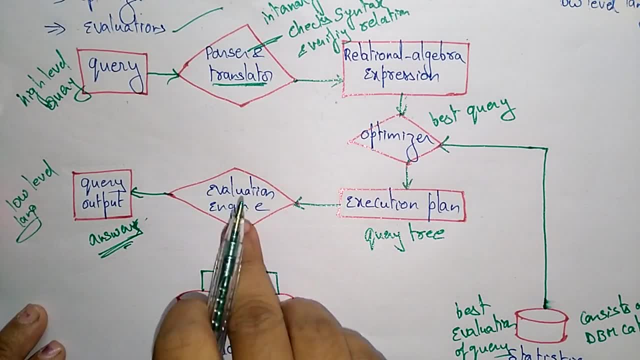 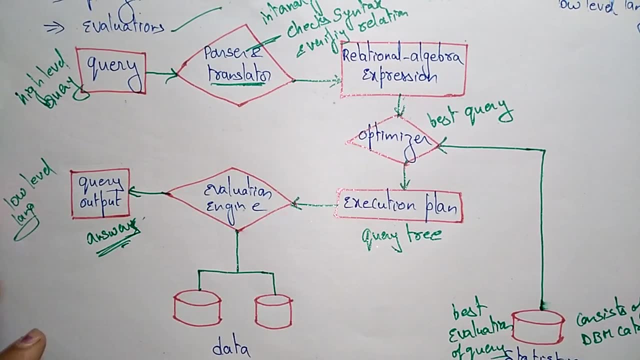 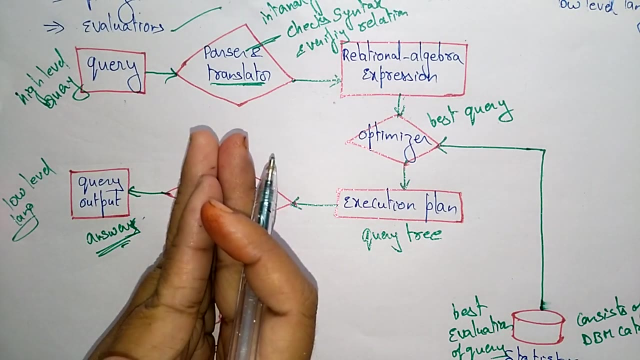 okay, so it will store course in this data and this evaluation engine takes the best one and whatever the next data that will be placed on the query output. so this is a query processing overview. first it takes the query, okay. after that the parser and translator will convert the query into internal form and it 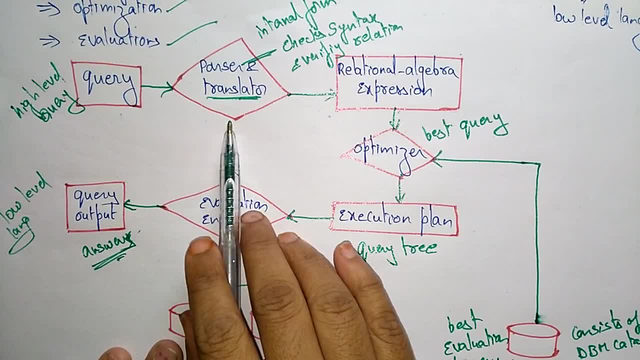 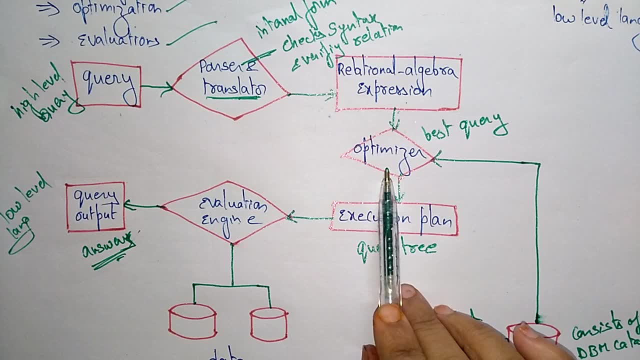 also checks the syntax and verify the relation, whatever the query that is, and it is converted into relational algebraic expression so that expression can be different expressions. in that different expressions, the optimizer will select the best query with the help of the statistics about data, which you call it as a DBMS catalog. so with the help of this DBMS catalog, it selects. 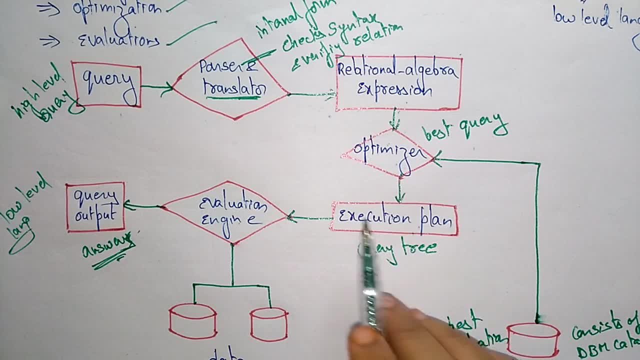 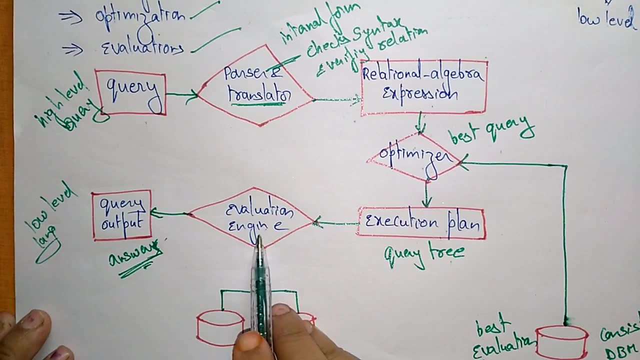 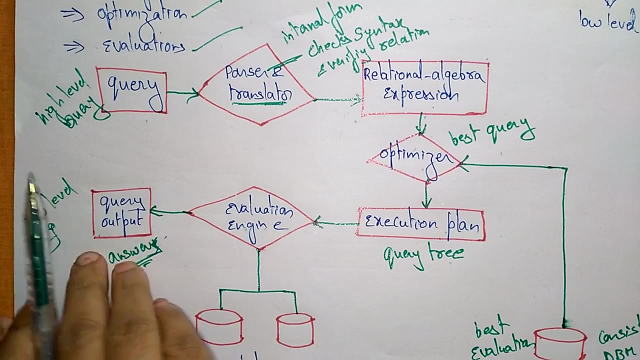 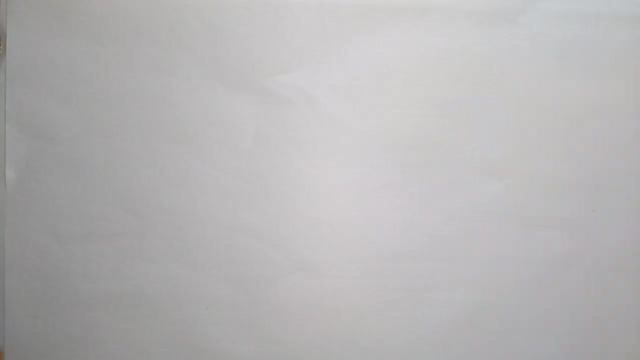 the best query and placed on the execution plans. okay, execution plan, convert that into form of query tree and it placed in the evaluation engine. now the evaluation engine will send that selected a query into the query output. so the here you will get the answer, the exact query, whatever we the database wants. okay, so let us take one example. 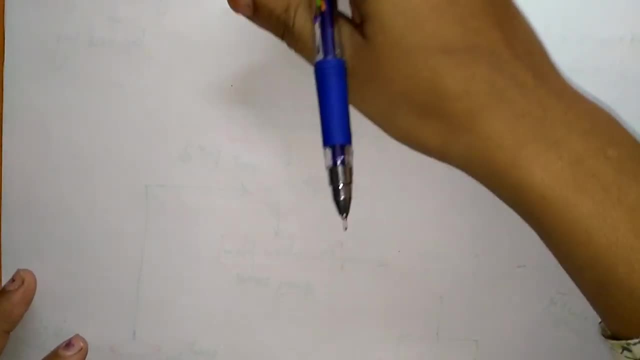 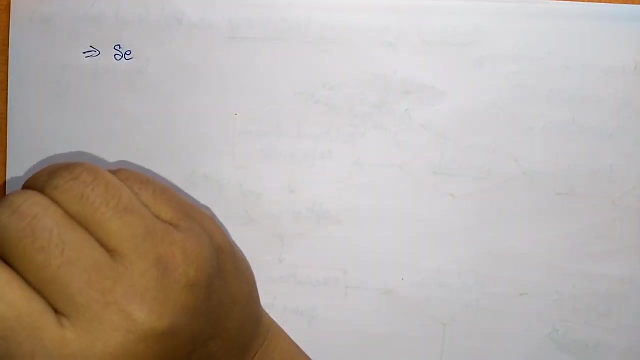 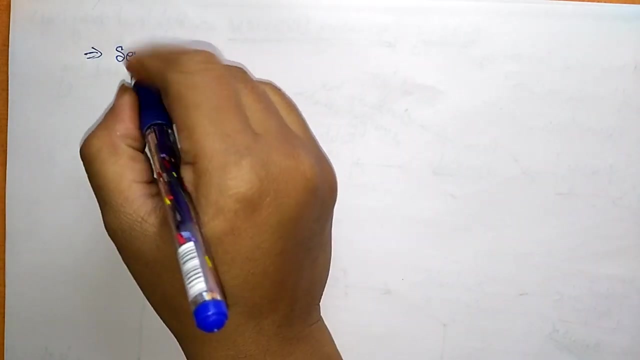 okay, so suppose the query is like: this means: first we are taking the SQL query. it's a high level query. so first, the query processor is a procedure of transforming with. I already said, it is a procedure of transforming SQL query to low-level language query. okay, so here. 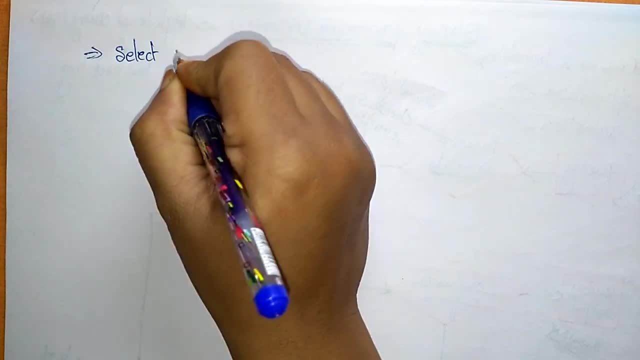 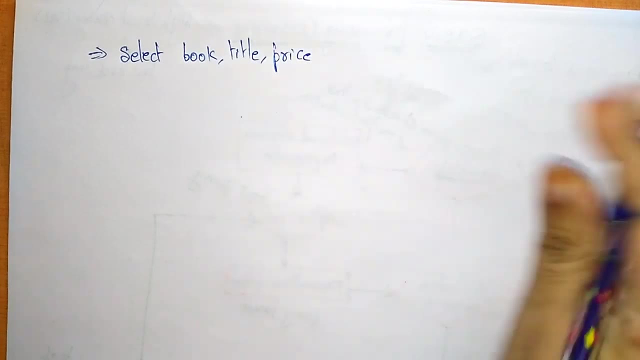 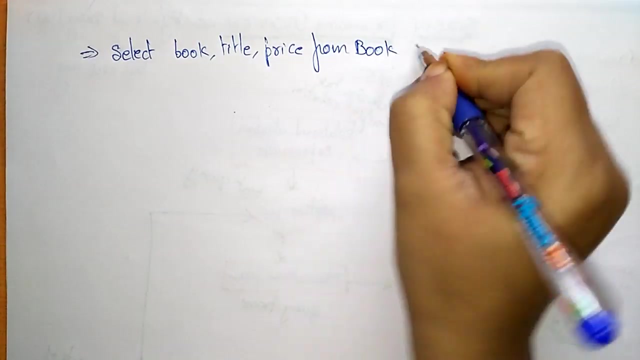 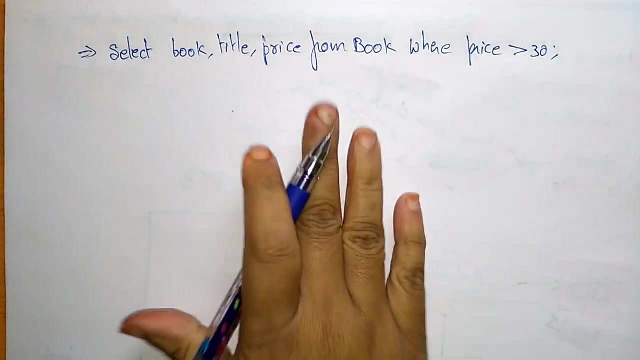 first we have take SQL query: select book title price. okay, select book title price from book where the condition is price should be greater than 30. so this is the query, this query we have to select, as a best query means one best query we have to be selected. 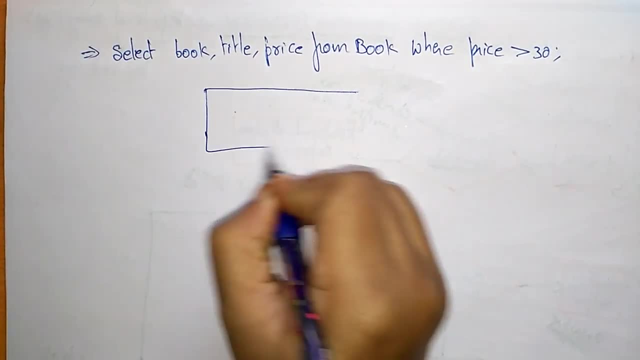 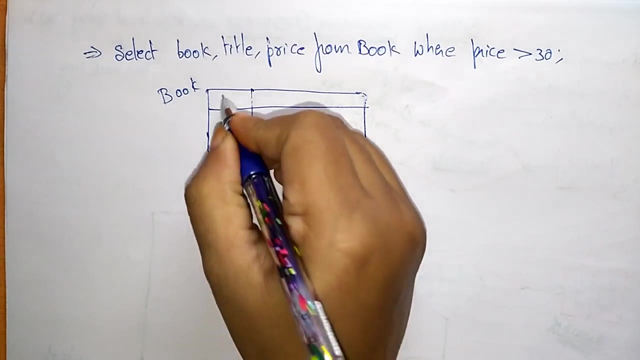 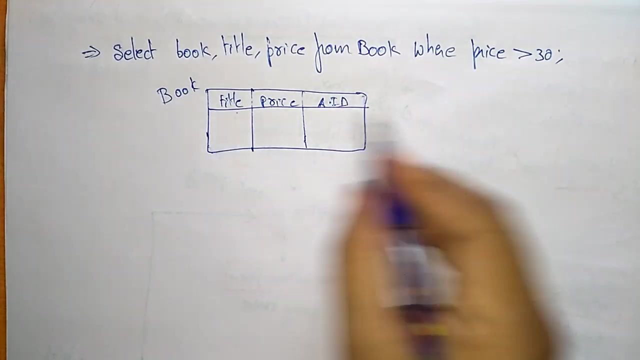 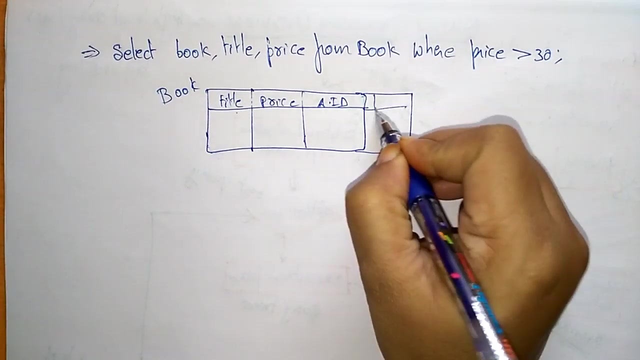 here you are given. a book is a table name, so book is a table name. in the table we are having the fields like title price, like author ID, so many fields are there. so in this table we are just selecting the book. okay, so book is also another field. so in this title book we are selecting the book title. 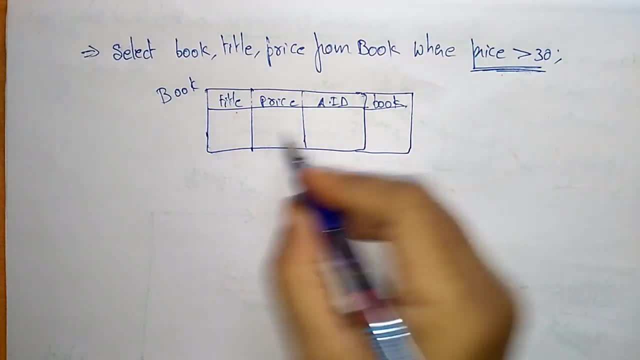 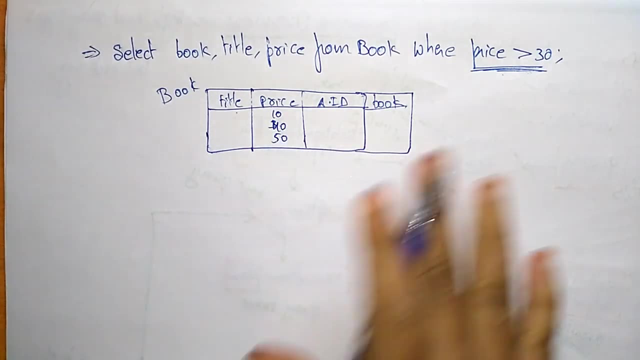 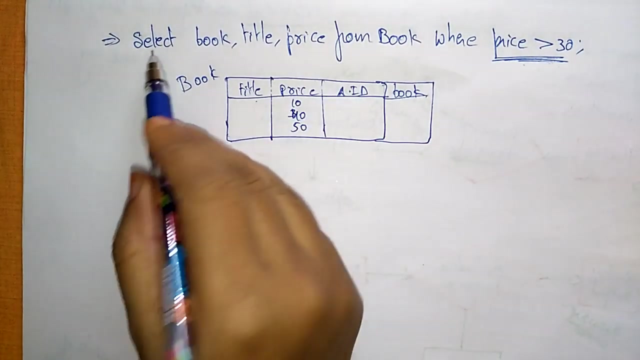 price. where the condition should be: the price should be greater than 30. okay, 10, 30, 40, 50 like that. okay, so we have to select the price that should be greater than 30. so first we have to do whatever. the SQL query checkbox will be converted into relational. 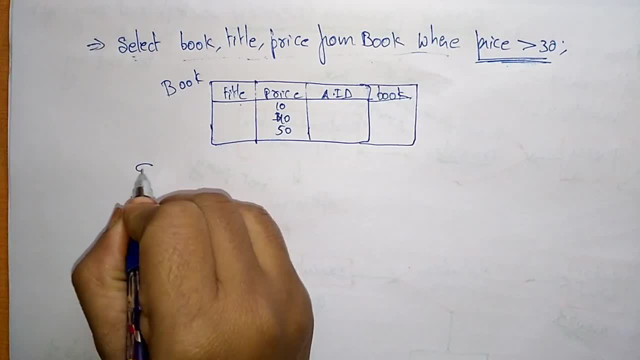 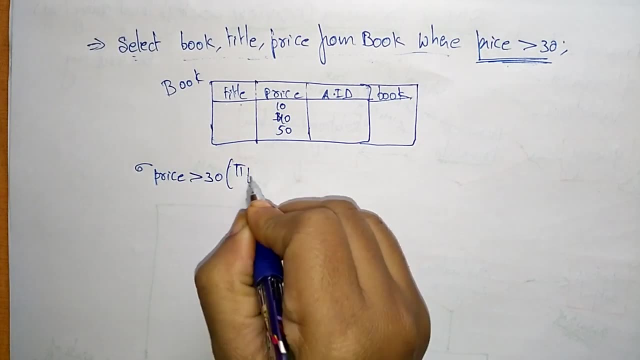 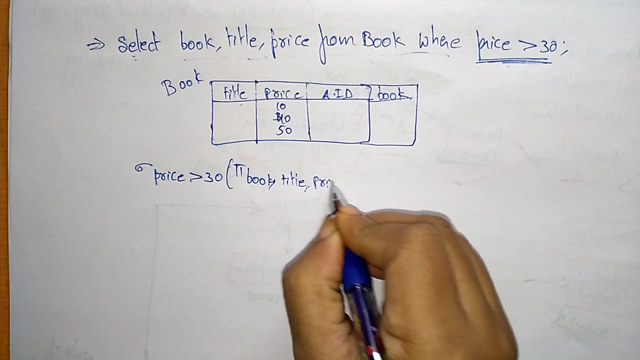 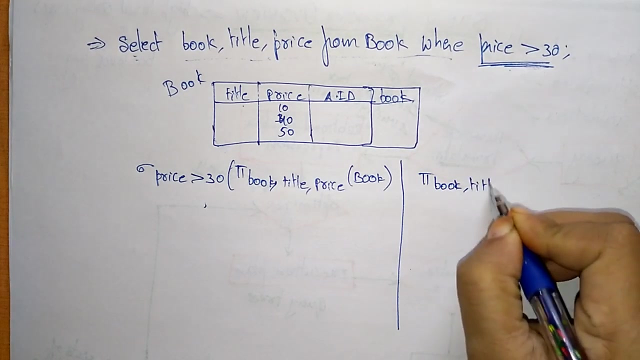 algebra. okay, so in this table we will write: price is greater than 30. UK Ottרה book that is split by title price. what we have to do, whatever the SQL query to respond to the query inica, or else you can write by book title price where price is greater than 30. 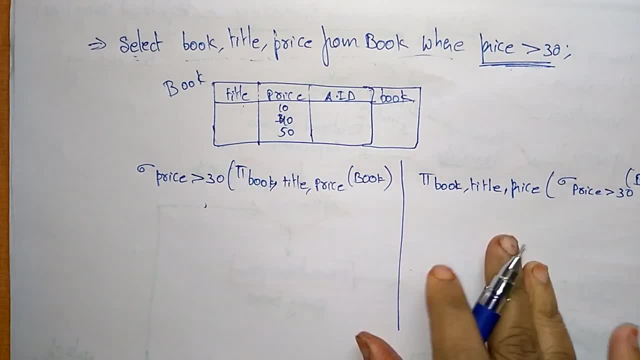 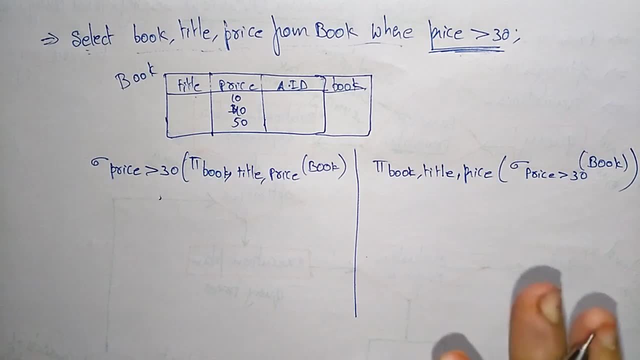 from the table book. so these two conditions, both these two expressions are same. the you will get the same output. but in this to we have this query optimizer will select the best query and place it in the evaluation engine. okay, so this will be first what it does. so the query evaluation engine- sorry, the. 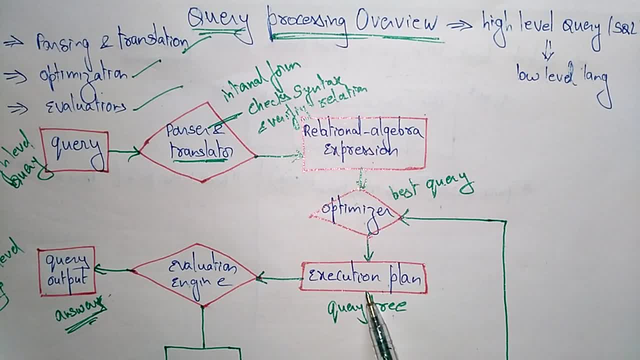 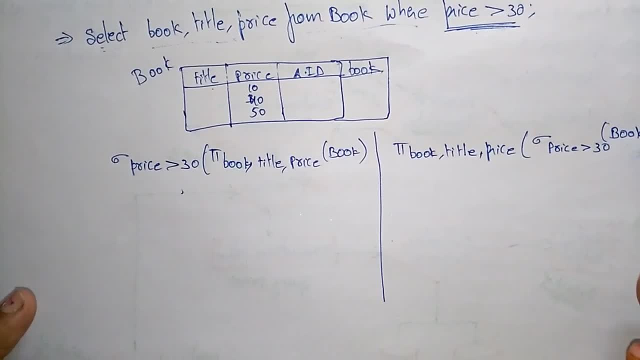 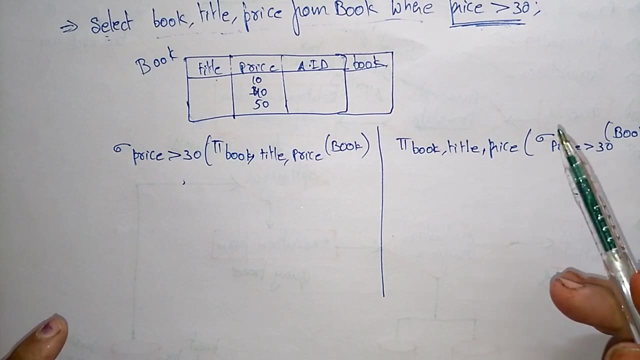 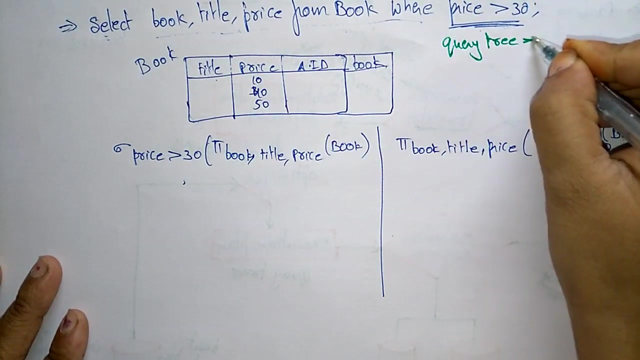 query optimizer will place the best query into the execution plan. so execution plan will convert that queries into query tree. okay, what is query tree? query tree is nothing, but it is used to represent the relational algebra expression. okay, so the query tree represents into relational relational algebraic. 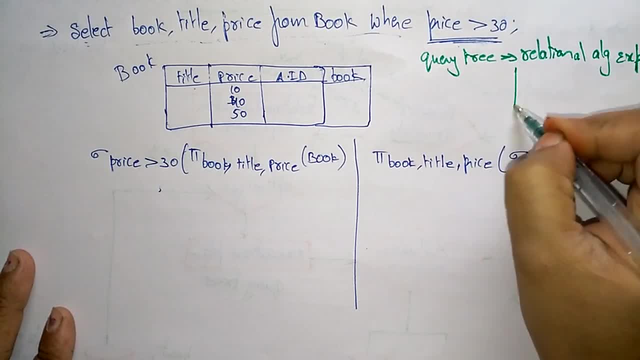 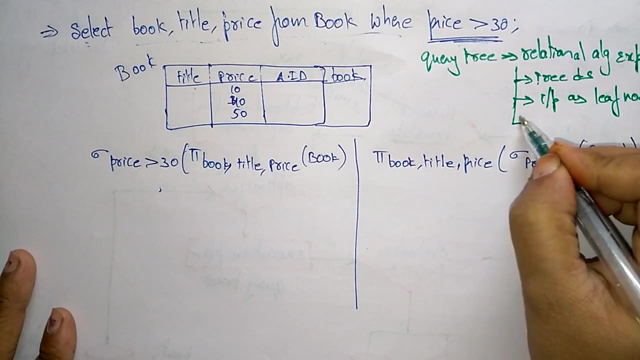 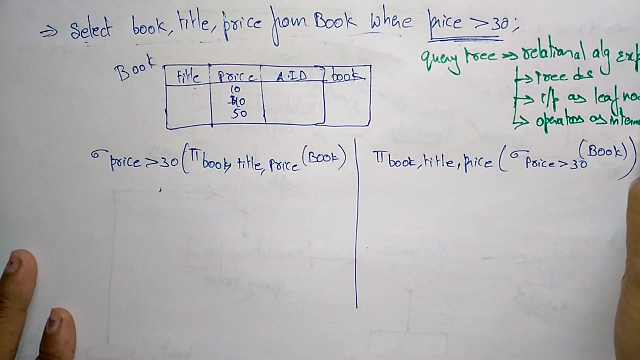 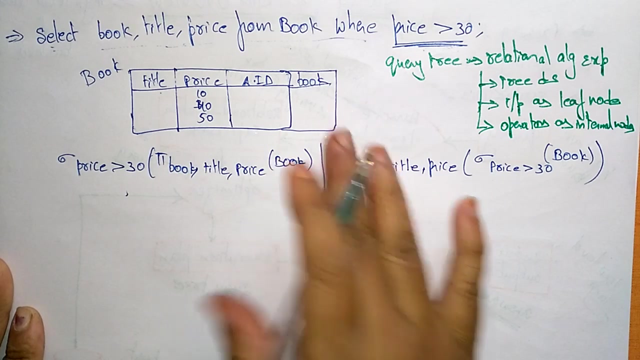 expression: okay, so that expression should be in tree data structure. okay, and all the inputs- relations- are represented as leaf nodes. okay, and the and all input represents relations are represented as leaf nodes and the relational algebraic operators and operators as internal nodes. okay, so this will be the conditions. the query tree is used to represent the relational 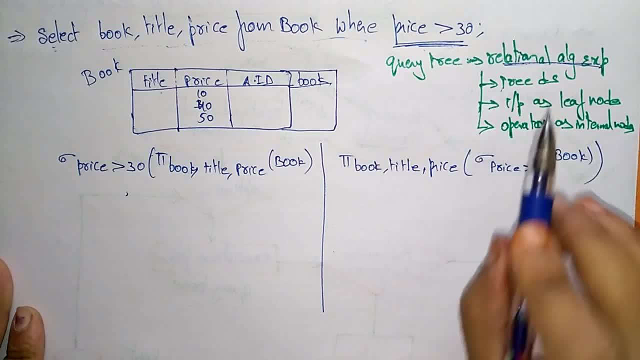 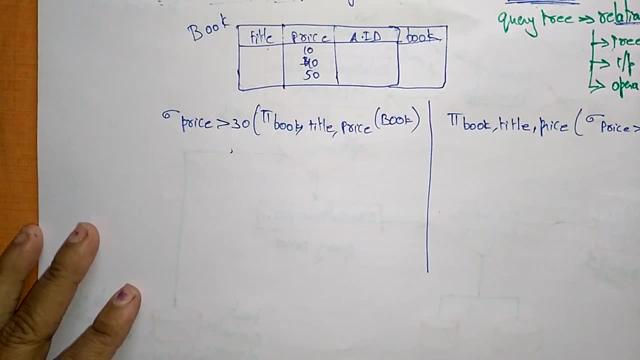 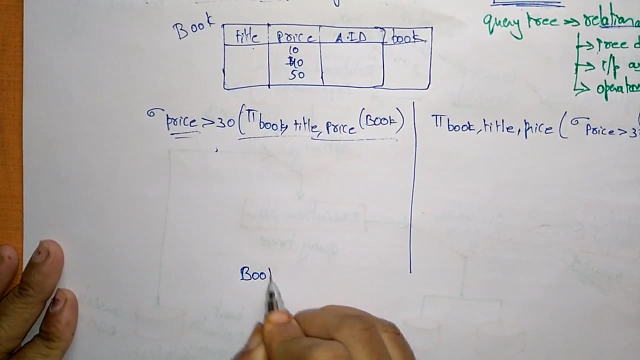 algebraic expression. so it comes. it is in the form of tree data structures, the Lee, the input is as leaf nodes and the operators will be used as an internal nodes. now let us see the query tree. so this expression will now convert into query tree. so first take the book, okay, so after that you have to take this. 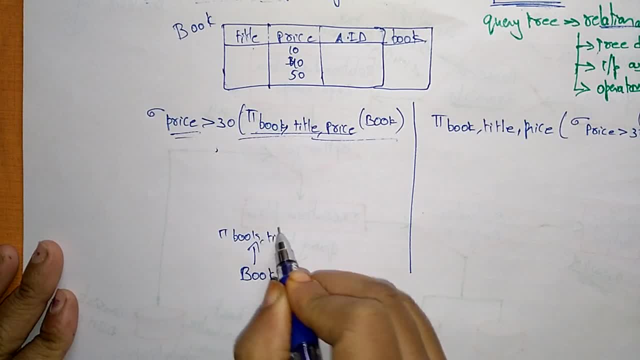 expression: PI book comma, title, comma, price. okay. after the the expression main explain: PI price greater than 30: okay. so any Boolean violation of B is来 home containing first place. sure that we have to get one must be fair, so we'll just go on to the provision. later. this another way you can claim it. in addition, it's just sort of journey- sorry, God is gonna be one, two, three. We want to get the pointer Here, one and go on to accept it and go in the application, as you have to go to the. 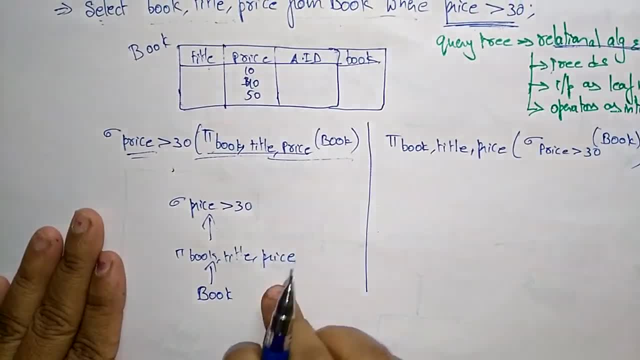 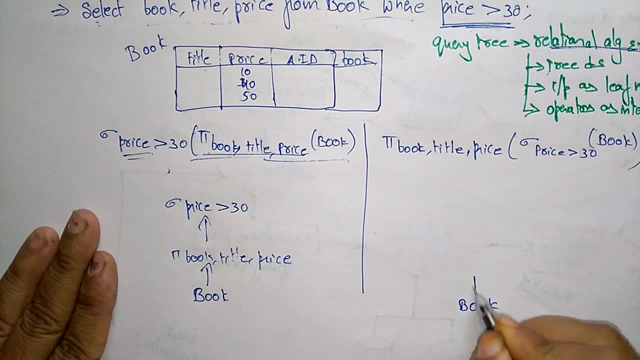 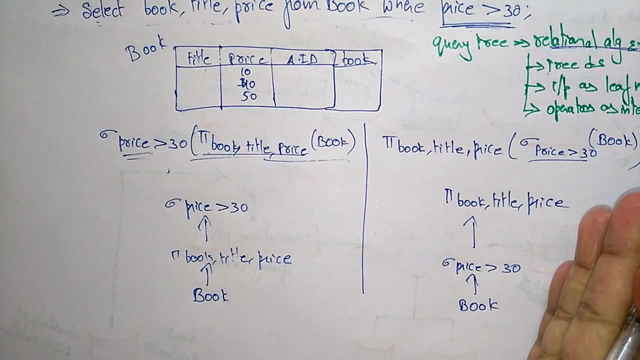 so this is the one way of representing the expression, this expression, in query tree. now coming to this expression. so the first one is the, so every book. next it's calculating the price. that should be greater than 30. okay. next pi book, comma, title, comma, price. okay, so now the query optimizer will check these two relations. relational algebraic expressions.